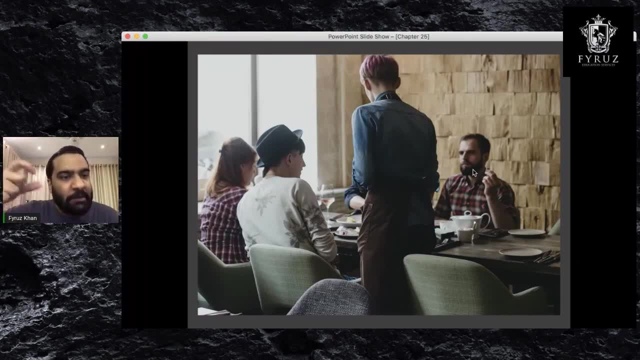 maximum capacity, or the maximum number of customers they can fit, is 150.. That's your maximum output capacity. You can fit in 150 customers, 150 diners: 150 people can eat at once at one go. That's your. 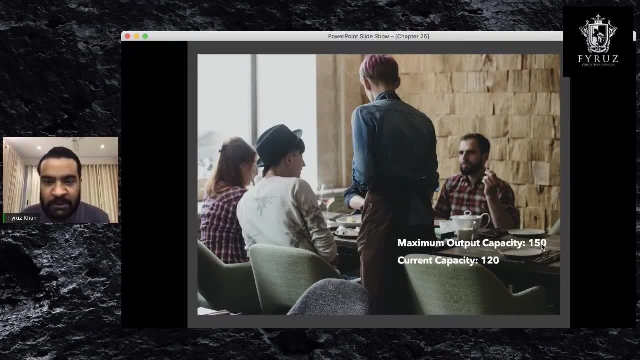 maximum output capacity, And your current capacity is: how many people do you have every day for dinner or lunch, or how many people visit you every day in your restaurant? Your maximum capacity is 150, but every day you have 120 customers. That's your current capacity, So you're using how much. 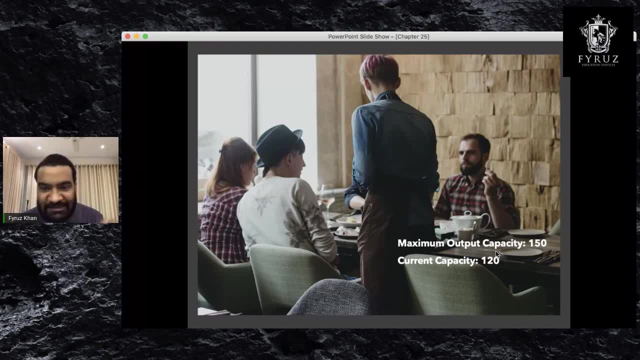 you're using out of your maximum capacity. It's 120.. You can fit in 150 people, but at this moment you are feeding 120 people every day. That's your current capacity And your spare or excess capacity is the seeds that is left Because you're not running at full capacity. Running at full capacity. 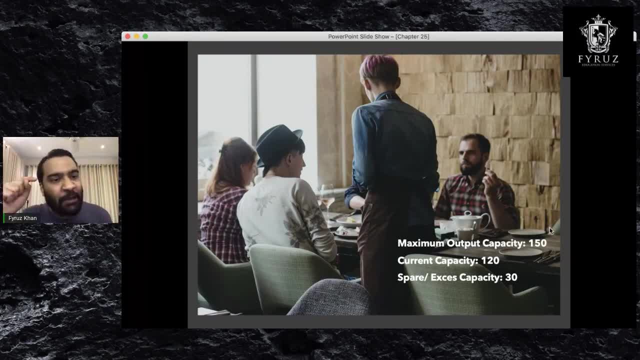 means if I have 150 seats, I will feed 150 people. That's running at full capacity. But we are not running at full capacity here. We feed 120 people every day. So the spare capacity if you just subtract, very simple. 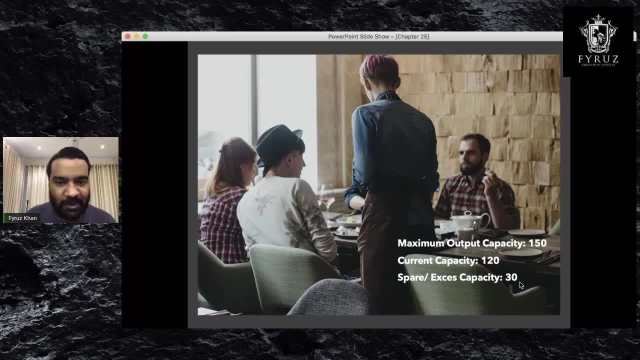 if you just subtract, it's 30.. Okay, that's your spare capacity. Now, if you want to know that how much, what is the percentage of your capacity utilization? you can easily. you can easily find out, It's so easy. So what you can do is 120,. okay, take the current capacity that you do. 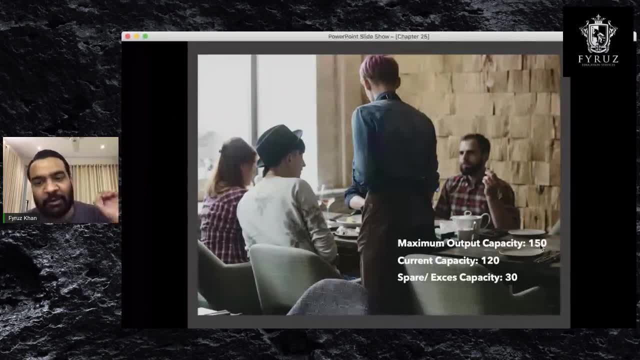 every day. take that, divide it by maximum output capacity. What is your maximum capacity? 150 into 100. And that is 80%. So out of 100%, you're using 80% of the restaurant seats every day. So that is your capacity, So 80%. 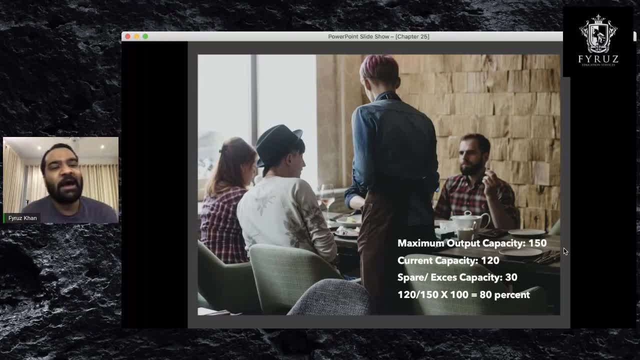 Is a good number. Okay, out of 100%, you're using 80% of your production facility. That's good. you're making good profit. you're using more of your resources, So that is a positive number. Okay, so your maximum capacity is 150.. That's the total people that you can have in your restaurant. But 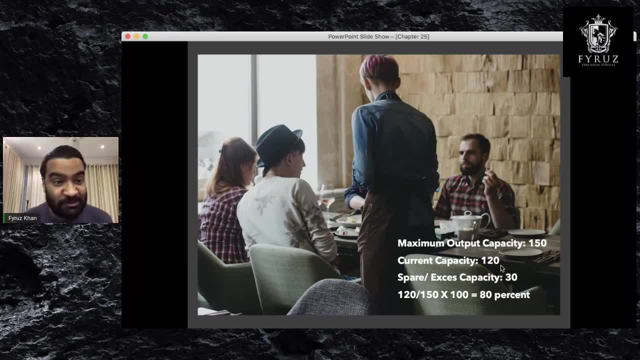 currently you're feeding or you have 120 customers, So that's not full capacity. Okay, full capacity means if we, if we feed or if we have 150 people every day, then we will be running at full capacity. But currently it's not, So your spare capacity just minus 150, minus 120.. The number of seats: 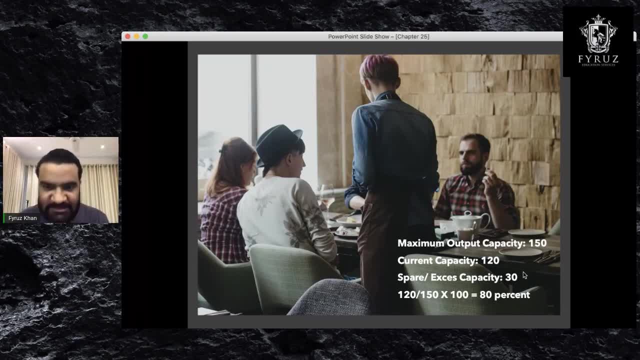 that's left every day. that's 30,, 30 seats, And you can find your percentage by simply 120, your current capacity divided by maximum output capacity, which is 150, into 100.. At this moment, this restaurant uses 80% of the seats, which is a good number. which is a good number. 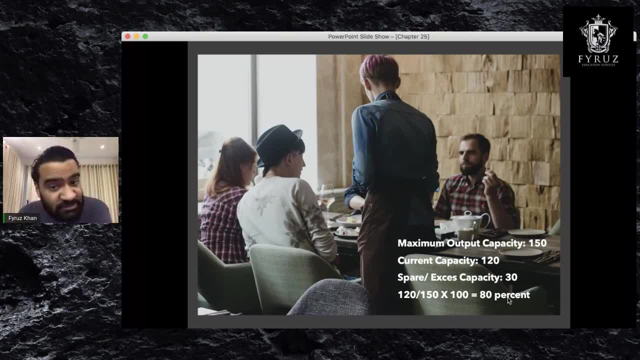 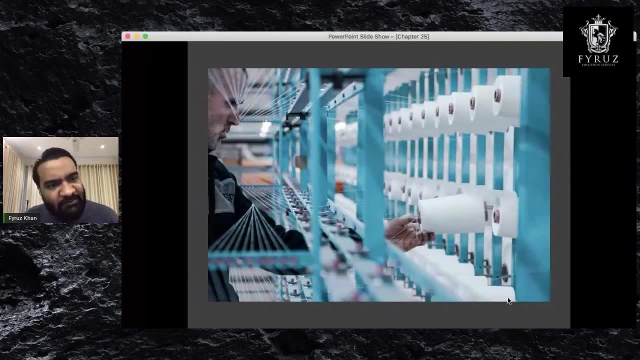 not bad. So they're using 80% of the resources. Now let's go ahead. let's have a look at one more example. We will have a look, we will look at more. let's say the industrial side. Let's say: 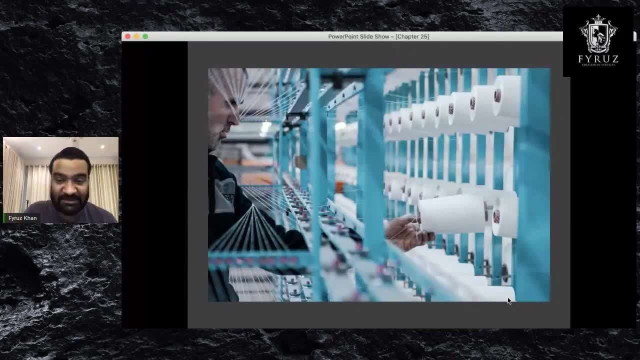 you're a textile factory. let's say you have a textile factory And your maximum capacity is: look here, look your maximum output capacity. let's say it's 150 tons or 150 metric tons. that's what you do, That's much. that that's how much you produce every day- thread or clothes. 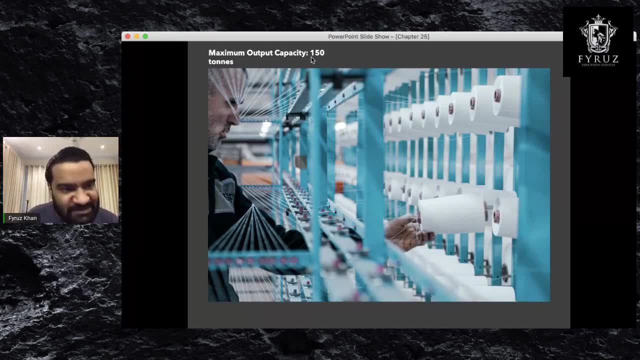 anything. Okay, that's your maximum capacity: 150 tons. Now, what is the current capacity? How much are you producing at this moment? This is what you are capable of At this point. you're doing 150 tons. you're capable of 150, but you're doing 130 tons because that's the order that you have. So 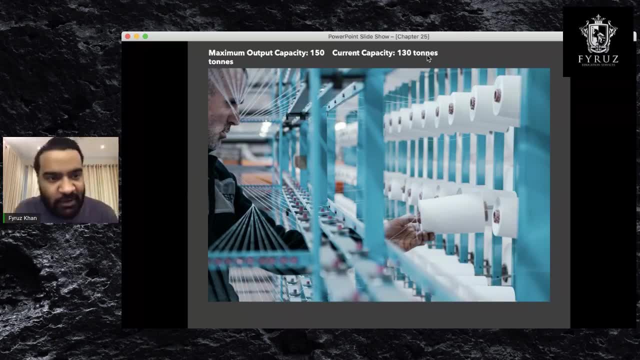 your spare capacity as you can. as you've guessed, from now, it's 150 minus 130.. That's 20 tons. Okay, now, if we have to find the, the current capacity percentage, we will simply take 130, divide by. 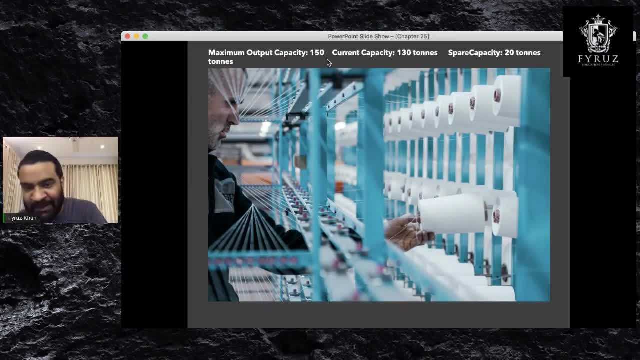 150 into 130. And and that is 87%. So this factory uses 87% of its resources, which is good, which is again a very high amount, more than more than the restaurant that we've compared. Okay, so so it. 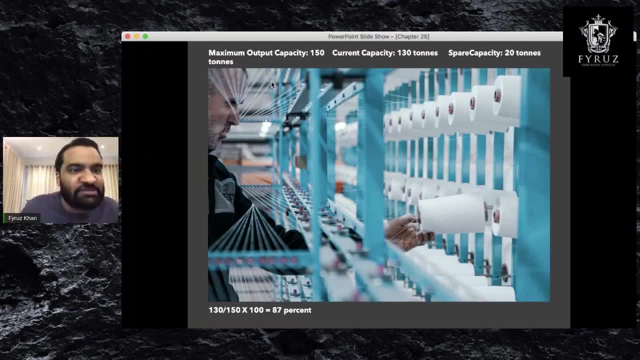 is a good amount. Now, the more capacity you use, the better. it is why we will talk about it. but then there are disadvantages also, But this is the chapter about it. So let's talk about the first thing, about capacity utilization. So what it's about? it's about capacity utilization. Okay, 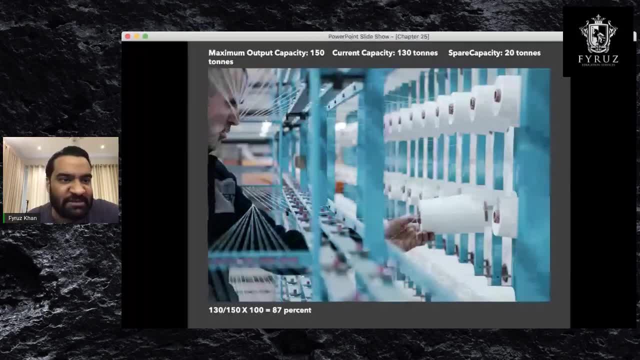 If you have any questions, please do not hesitate to comment on the section here. Type in on our page. FIRO's Education Services. If you comment on FIRO's Khan profile, I will not be able to see, So make sure you comment on FIRO's Education Services So I will be able to see. There's a problem with. 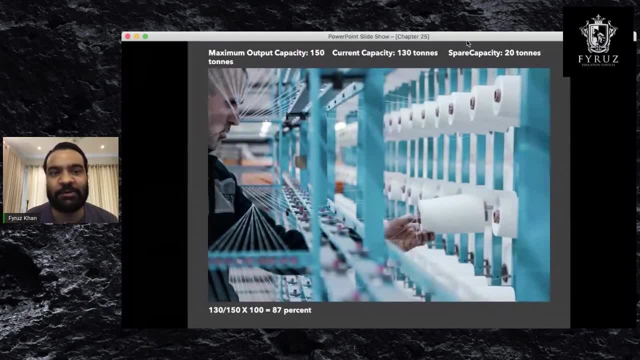 the system. I'm trying to fix the comment thing here, but then yeah, So this is what the chapter is. dyslexiacom. So this is what the chapter is. this is: how can we use FIRO to get it working? 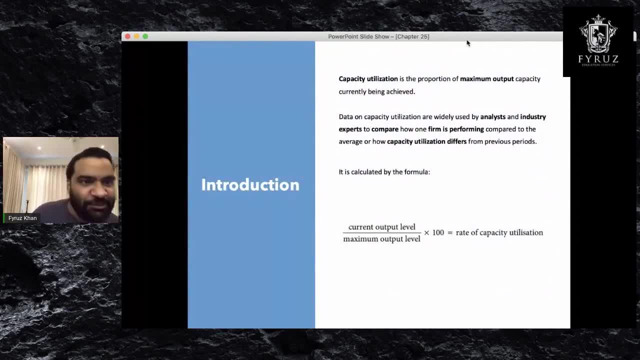 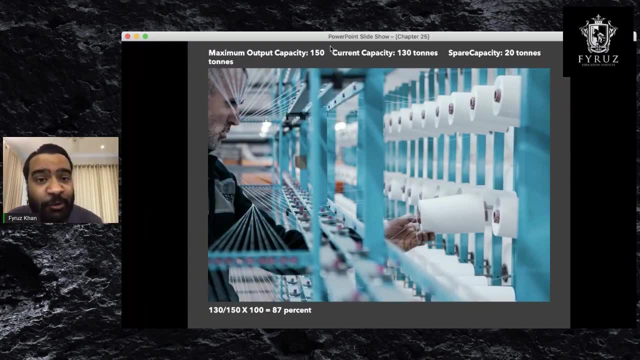 chapter is about. So capacity utilization is the proportion of maximum output. So what is your capacity utilization? We know maximum output is 150.. Your current capacity is 130 tons And if we want to find out the percent, this is the math that we need to do. So what is the proportion of? 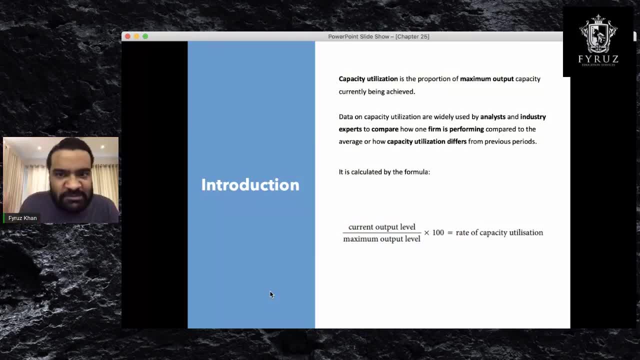 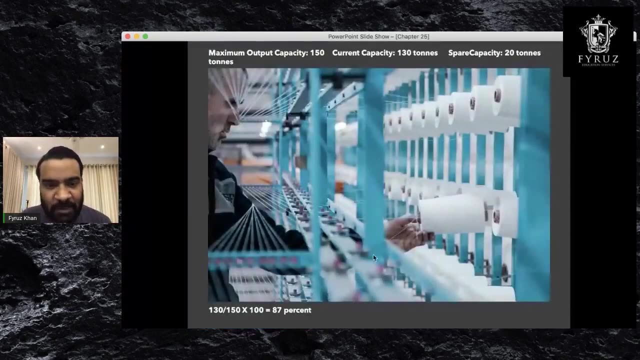 what is your? you know capacity is what is the proportion of maximum output that you do at this point? And this is the formula: Current output level divided by maximum output level into 100.. That is the rate of capacity utilization. So 87% is the rate of capacity utilization. 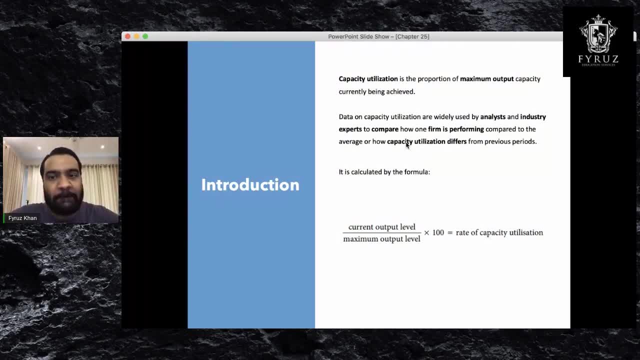 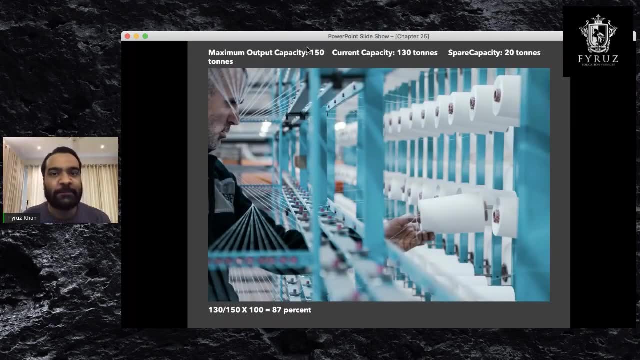 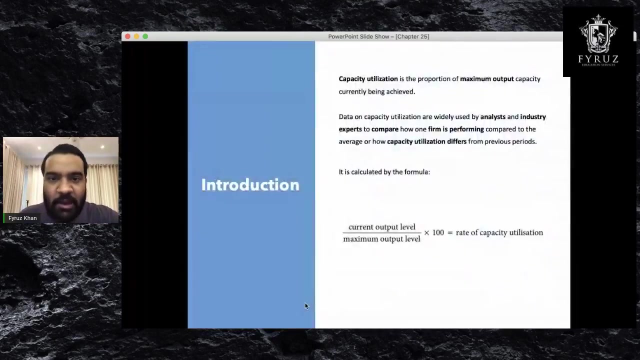 So capacity utilization is the proportion of maximum output capacity. So our maximum output capacity is 150 tons. Now what is our capacity? Our current capacity is 130.. Okay, So that is our capacity utilization And the rate is 87%. As simple as that. Okay, let's go ahead. 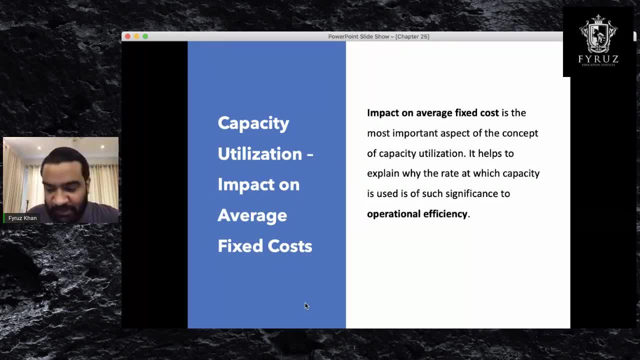 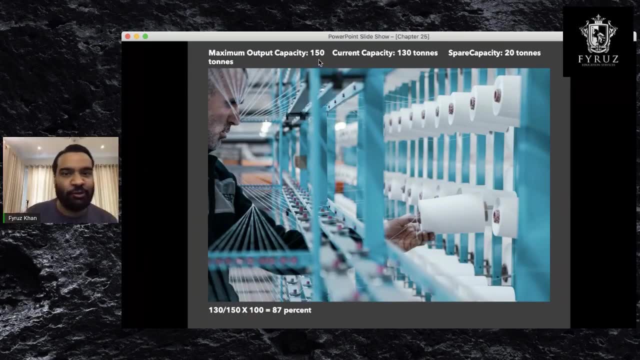 So there are two impacts that you need to think about, Because I told you that you know if you have full capacity utilization, if you, let's say, your capacity is 150 and you are currently operating at 150 tons, that's very good for you. You are at full capacity. If 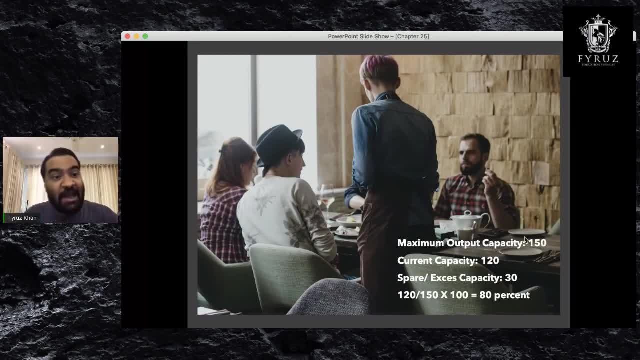 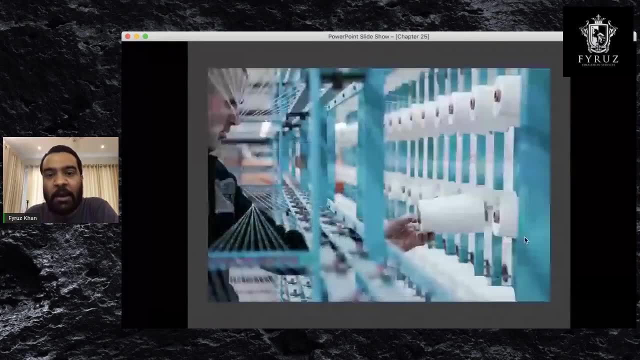 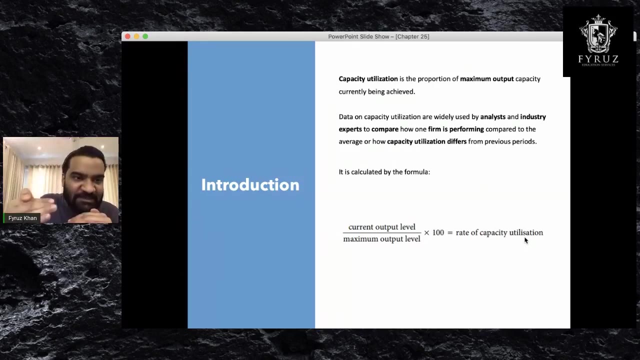 your restaurant has 150 seats and you are being able to feed 150 people. that is very, very good, because you're running at full capacity. When you run at full capacity, or when your capacity rate is high, when your capacity utilization is high, what happens is your average cost falls. 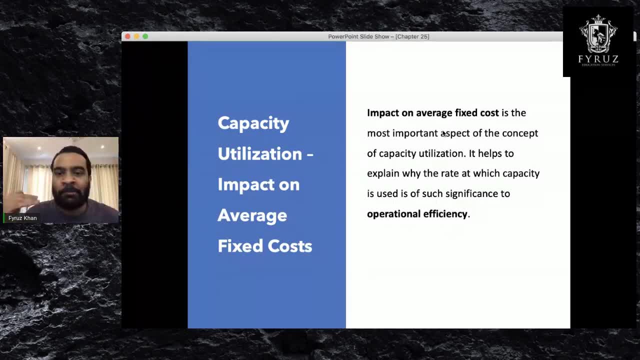 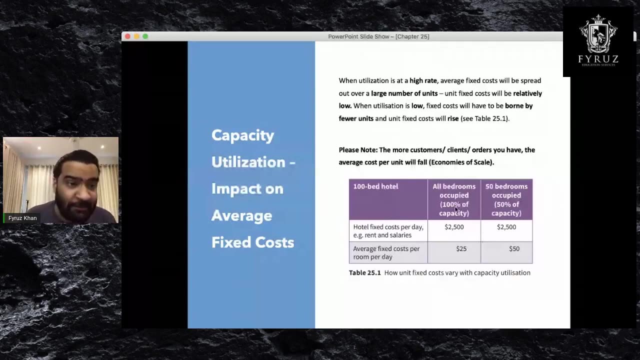 Your average cost becomes less. Again, economies of scale. The more you produce, average cost per unit will fall. So that's what impact on average cost? Average cost will fall. We will have a look at one more example again. Think about a hotel which has 100 rooms. 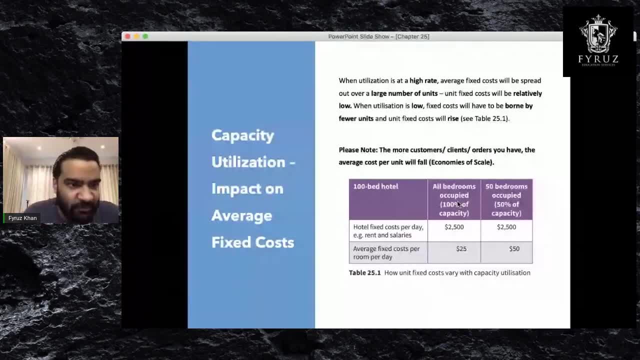 Now, in any business you have a break-even point every day or every month. Let's say, break-even for this hotel is $2,500.. Whether you run at full capacity or whether you don't run at full capacity, whether your rooms are fully booked or half booked, every day 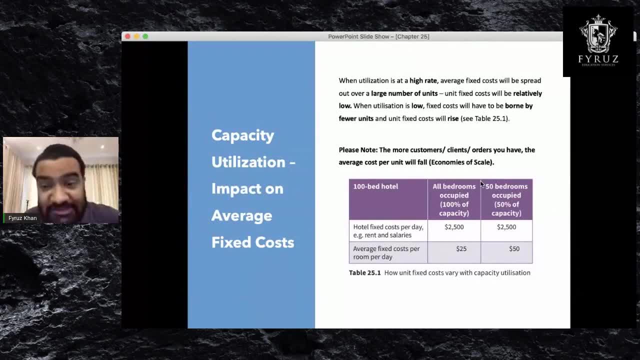 your fixed cost or your cost is $2,500.. So that's a lot of money. So when you're running at full capacity, you have a break-even point every day or every month When 100 rooms are occupied. let's say, in a very good day when 100 rooms are occupied. 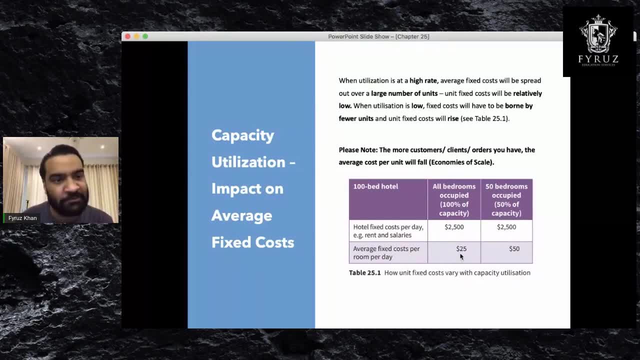 your average cost is $25 only. But if your hotel is half booked, if only 50 rooms are booked- just look at this- If only 50 rooms are booked out of 100 rooms, then your average cost it rises to $50 from $25.. 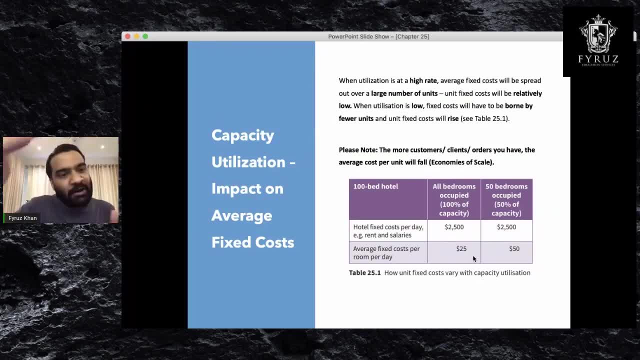 We can guess from here that the more busy you are, the better it is for average cost. If you're running at full capacity, then what happens is your average cost will fall down. So it is $25 when all 100 rooms are booked. 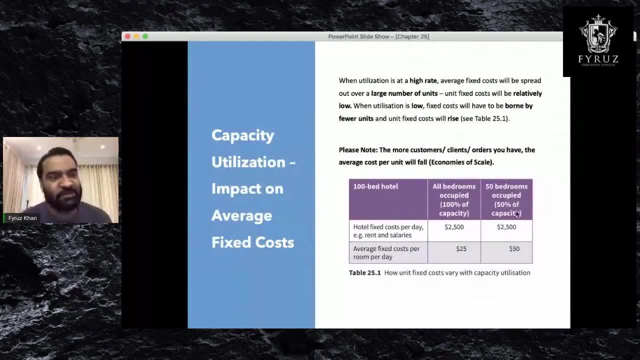 And when only 50% of the rooms are booked, it's $50.. So note that the more customers you have, the more clients you have, the more orders you have. the average cost per unit will fall, And this simply relates to economies of scale. 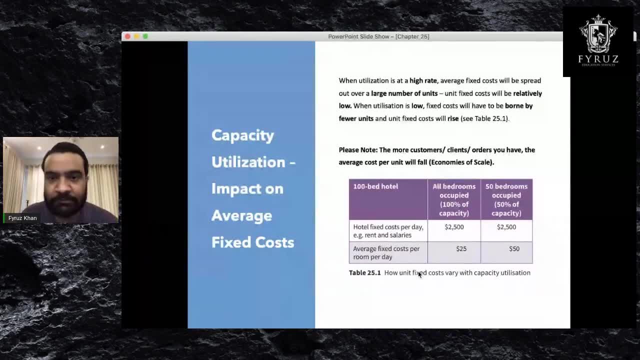 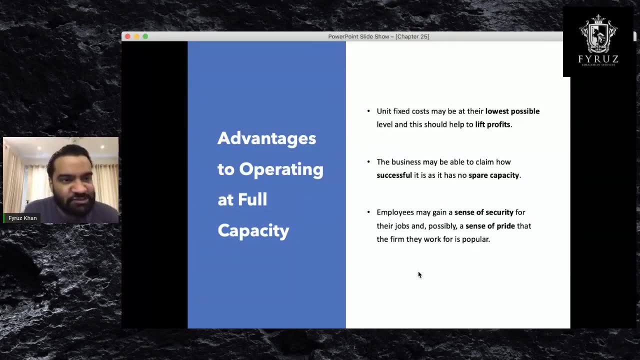 Okay, there we go, Economies of scale. So think about that. So what are the advantages of running at full capacity? So if you have 150 seats- let's say all your rooms are booked- then your average cost will fall down. And if you're running at full capacity, 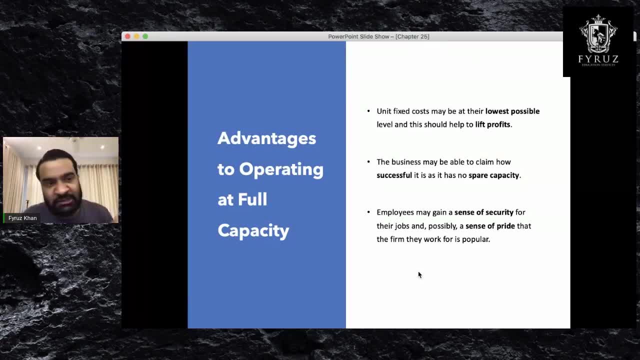 let's say, all your 150 seats are booked. if your production capacity is 150 metric tons, that's all you are producing 150 metric tons. What is the advantage of that? The first advantage is unit costs will be very low and you will 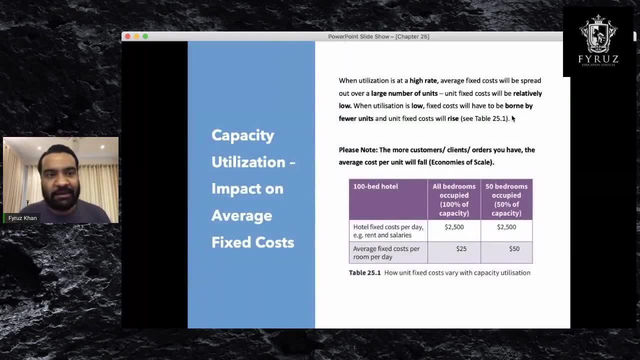 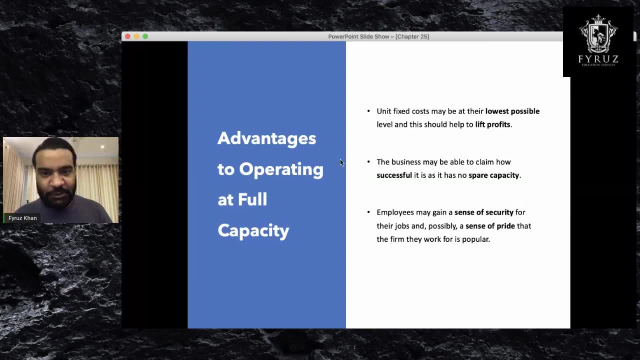 make more profit And we have seen that from this example right. So unit cost will be very low and you can also say that you know we are very busy and that means you are successful, And that means you are successful. 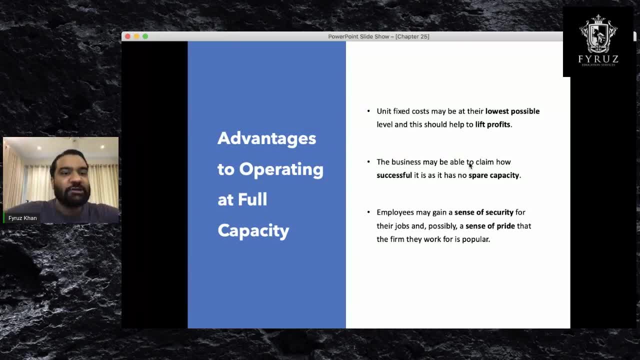 That means you're getting more orders, and getting more orders show that, as a business, you are successful. The second point, OK, the third point is there's a sense of security, There's a sense of pride that you guys have worked. You know the workforce, the employees will be motivated. 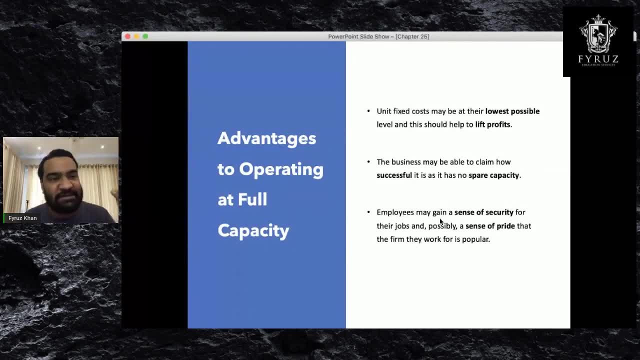 There'll be a sense of security, a sense of pride. So these are three advantages of operating at full capacity. The cost will be very low, You will enjoy economies of scale because you're running at full capacity and therefore you'll be able to make more profits. 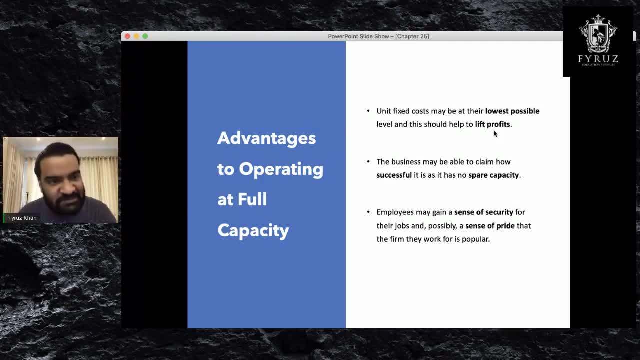 Number two: it shows that as a business, you are successful. Number three: the workforce. the employees will have a sense of security, will be motivated because they have lots of work to do. So these are the advantages of operating at full capacity. 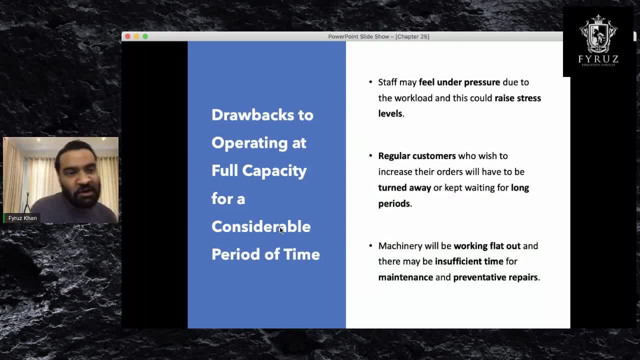 Now there are drawbacks also. If you have 150 seats, you're booking, you're taking 150 seats every day. That also has a drawback. What drawback does it have? Staff may feel under pressure every day. They have so much to do. 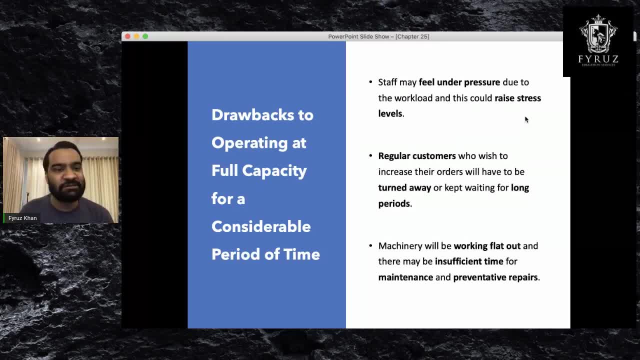 It may increase their raise their stress levels So they may feel under pressure. I used to work for this restaurant when I was a student in the UK. Every day it was busy. It was, I think, a 70-seater restaurant. They had 70 seats in the restaurant and every day it was fully booked And we used to be very tired when we got back home at 12 o'clock. So you know staff may feel under pressure. It may increase their stress level. 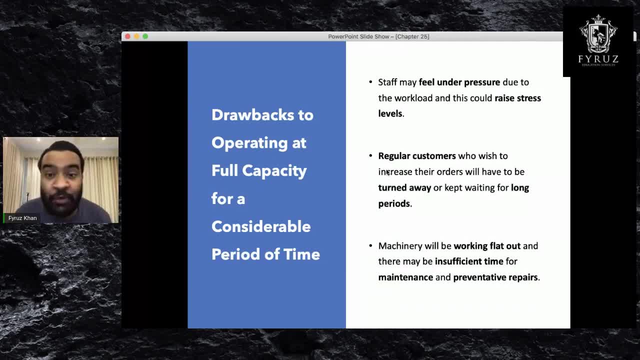 OK, sometimes the business may get too busy and regular customers may be turned away because the business is very busy, Right, Every day. every time Let's say there are, there is queue outside, you've seen businesses, right, You get demotivated. 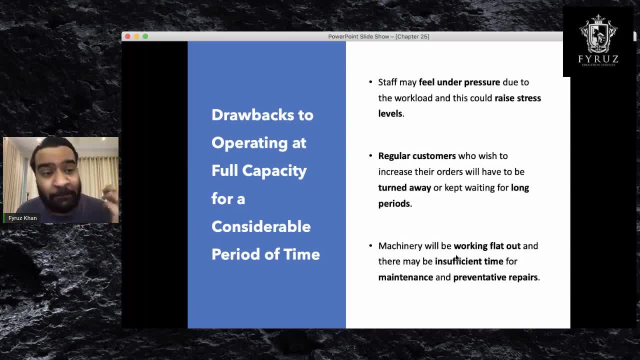 OK. And the third drawback is- and it's a very important drawback- staff machineries. everyone will be working flat out. You're not giving any kind of rest period. Now, if I use my phone 24 hours a day, it's not good for the device. 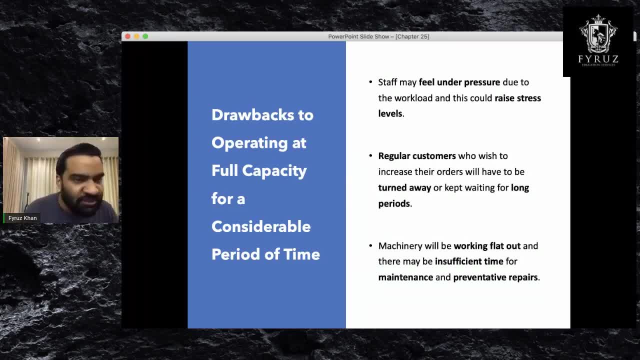 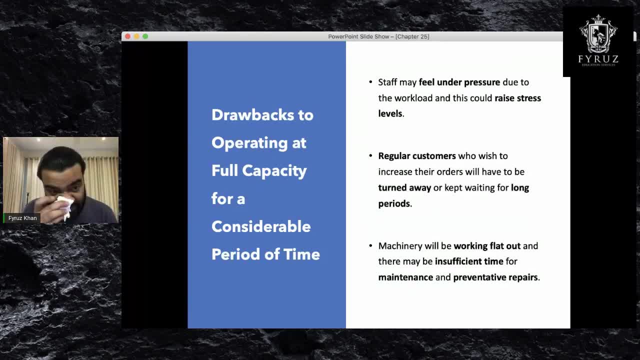 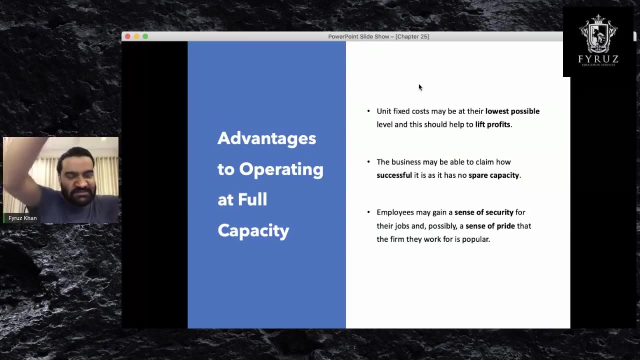 And that is not good. So that is the third. the third drawback that we can see, And you know, machines, they need repair, They need maintenance. So that's there. So three advantages of running at full capacity. Let's say you have 150 seats and you serve 150 customers every day. 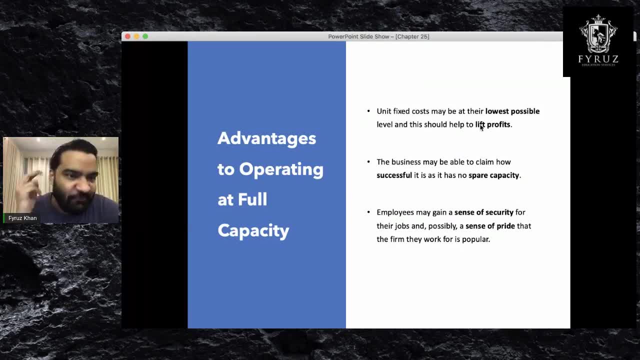 The advantage of that is unit cost will be very low Average unit cost. You will enjoy economies of scale. As a business you're successful. There's no spare capacity or excess capacity And employees will be motivated. They will have a sense of security. 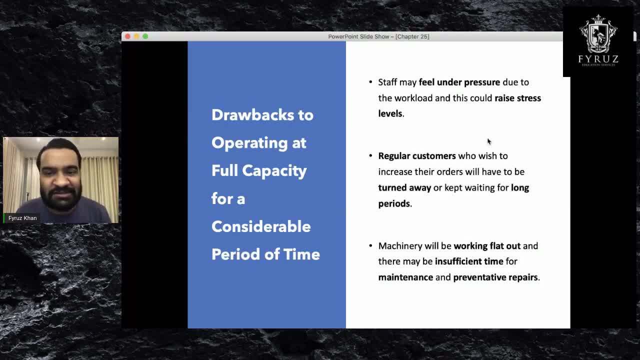 But, however, staff may feel under pressure, under stress, Regular customers may be turned away because you're so busy You can't take them. And third, machineries will be working flat out. You need to be able to run, You need to maintain them. 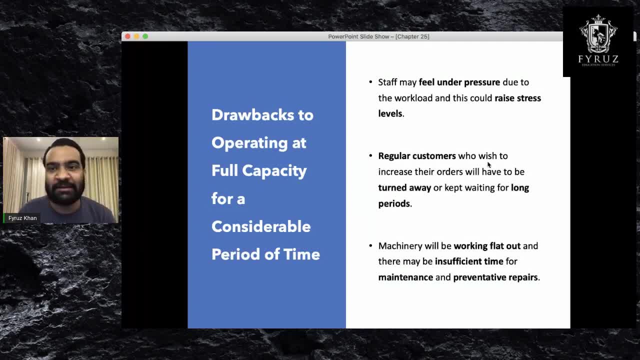 You need to repair them, Okay, So that's that. If you have any questions, please do not hesitate to comment on the comment section And I will be taking all your questions. And yeah, let's go ahead. So excess capacity. 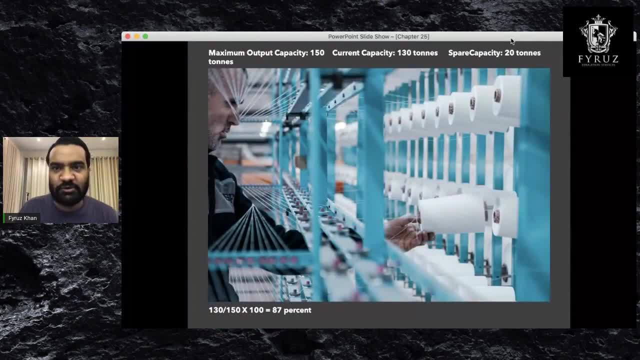 What is excess capacity? And we have talked about it here. So excess or spare capacity is, let's say, your maximum capacity 150.. Spare capacity is or current capacity. The capacity that you're producing at this moment is 130.. 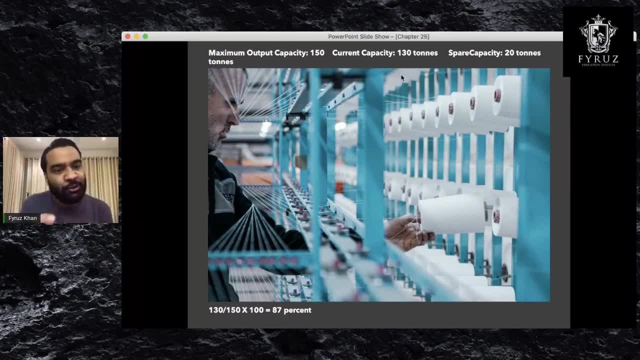 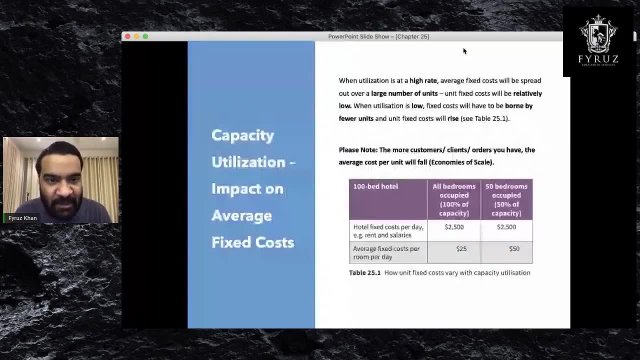 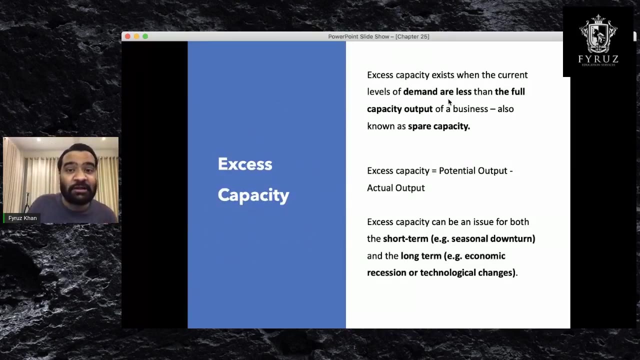 So your spare capacity will be 150 minus 130.. How much you can produce more? What is left after you produce. So that's your spare or excess capacity, Right? Excess capacity exists when the current level of demands are less than the full capacity output. 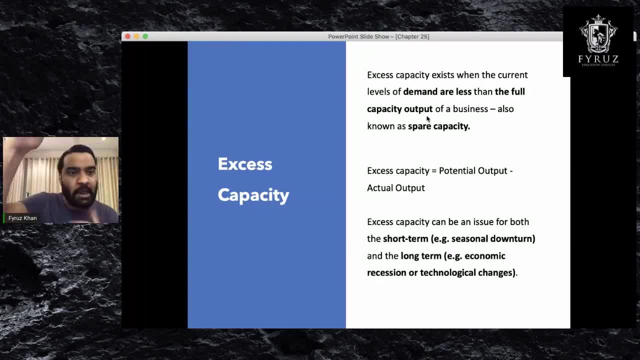 Let's say your full capacity is 150 metric tons, But your current level is less than that. Let's say it's 130.. It's 120, 110.. Okay, So excess capacity is potential output minus actual output. Potentially you can produce 150 metric tons, or you can have 150 customers, but now you have 110.. 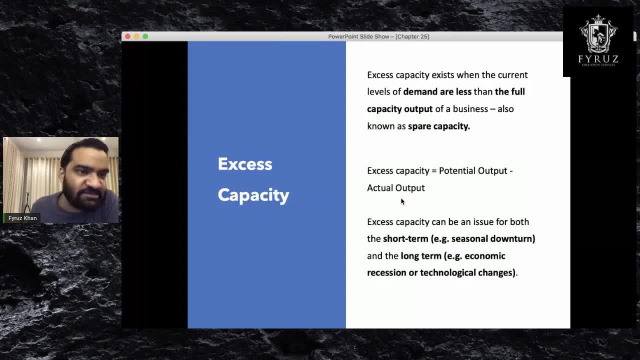 So your excess spare capacity is, you know, 40 or 30.. Okay, So that's that. And this happens sometimes. Sometimes, or most of the times, you produce under your capacity Because of, let's say, seasons, because it's summer break or because it's Eid vacation or Ramadan or Christmas vacation. 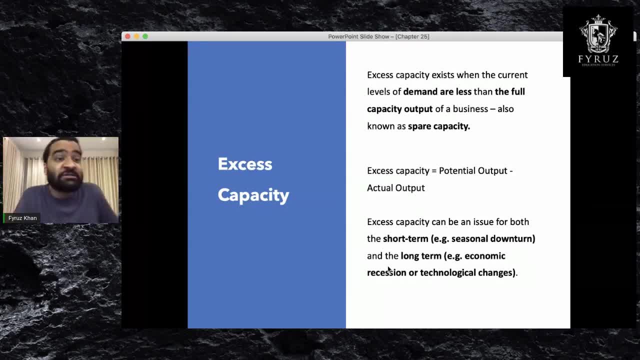 It happens Due to special situations like COVID-19.. Okay, It happens, Right. So there you go. So that's excess capacity. Now, if you have less excess capacity, that's okay: 10 tons, 20 tons, 20,, 30.. 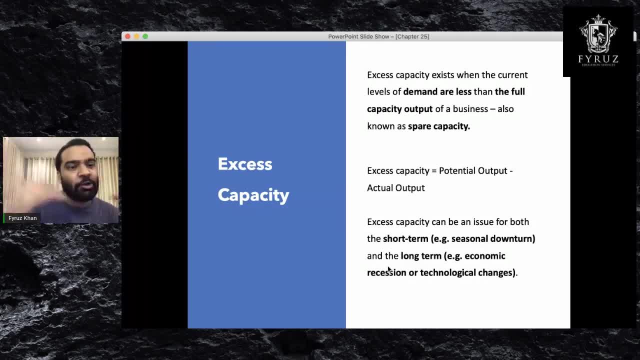 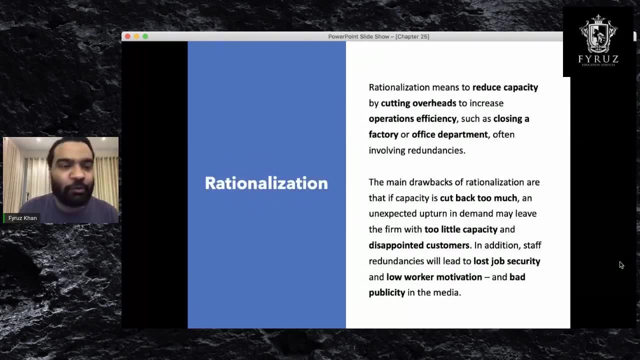 That's fine, But if it's beyond that, then it's a problem. Your cost will start increasing. So you have to be careful in a way. Okay, Let's go ahead. Rationalization is a concept which means you want to cut down overhead cost. 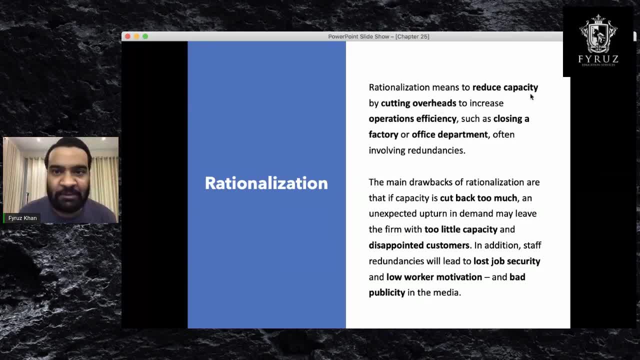 Sometimes you will hear in the news or you will hear your family members say that you know factory is closed. There are a lot of costs. You know workers. you know getting rid of workers or making the workers redundant. 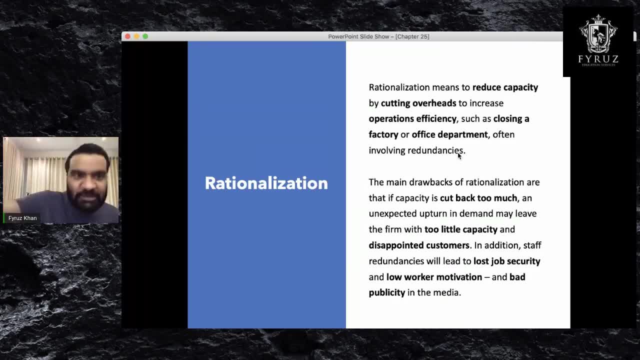 That is rationalization. Rationalization means cutting down cost. Okay, Because you want to focus on production. you don't want anything to go wrong. That's why you cut back on cost. You can cut back on cost is by getting rid of employees shutting down factories, shutting down departments or shutting down you know other sections. 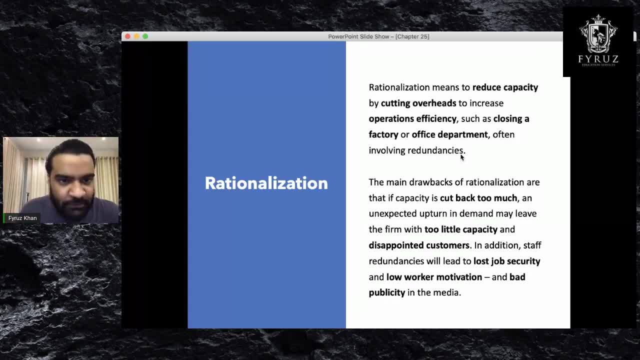 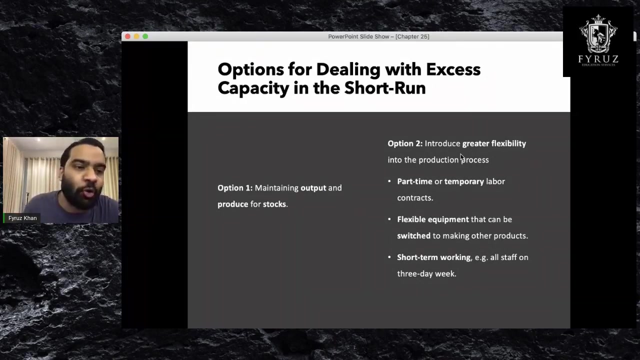 That is rationalization. Okay, And rationalization is used everywhere you know, to cut down cost, to make the production more efficient. So yeah, there you go. So that is rationalization. So what happens when you have excess capacity in the short run? 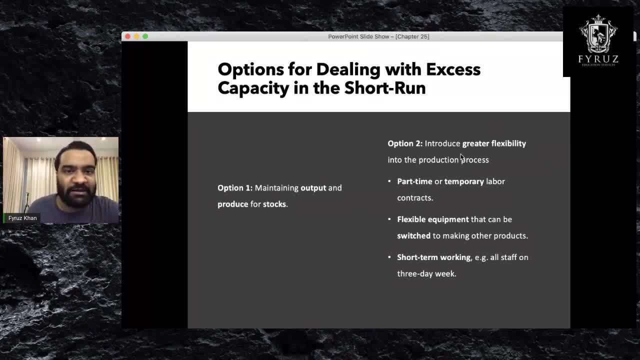 So let's have a look at some of the instances. Okay, Let's say, if you have, you know, if you have, let's say, your maximum capacity. Let's say your maximum capacity is 150 tons, but at this point you have, you know, 100 tons order. 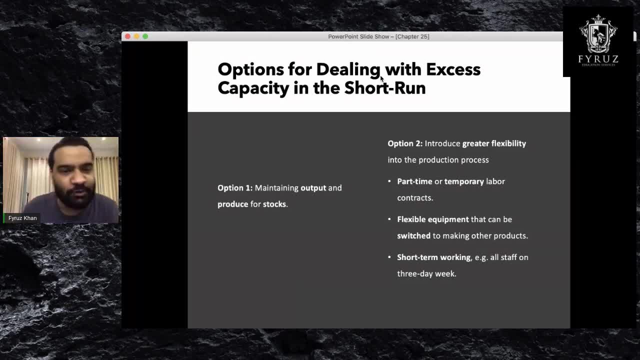 So you have an excess capacity of 50. So what do you do? There are two options. You can maintain output and produce for stocks. You can produce goods for 150 tons, Okay, And you can store them for later use to sell it later. 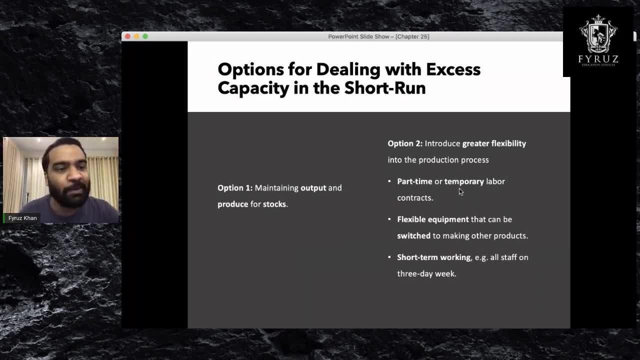 But option two. you can do option two, which is you know, hire part-time workers, produce others. You can produce other products. you have flexible equipment and produce other products. Or you work three days a week, You can also do that. 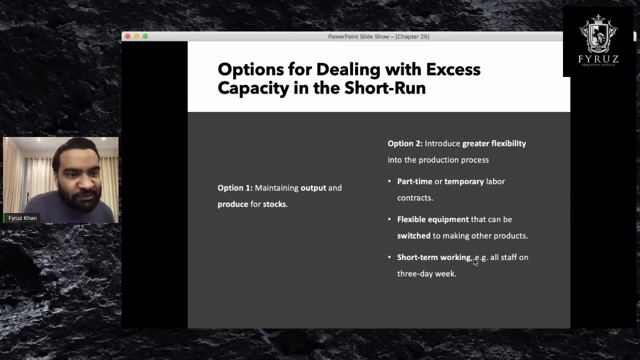 For example, a lot of pharmacy companies are not producing any kind of medicine. What they're doing is they're making masks, They're making sanitizers, Because people are not buying other medicines. People are focusing on these things because of COVID-19.. 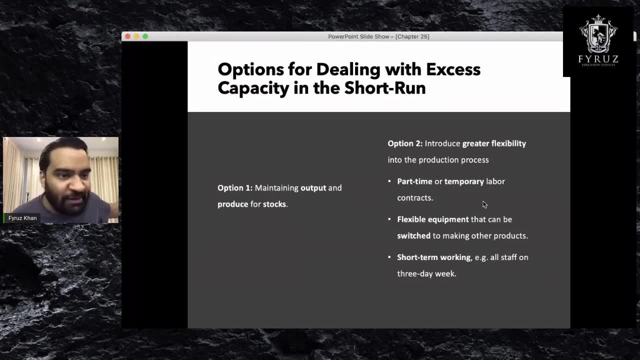 So, instead of making those regular medicines, you can make sanitizers, Because that is selling really well. So you have two options: You can either carry on what you were doing Okay, Because those products will be needed later on, Or you can hire part-time staff. 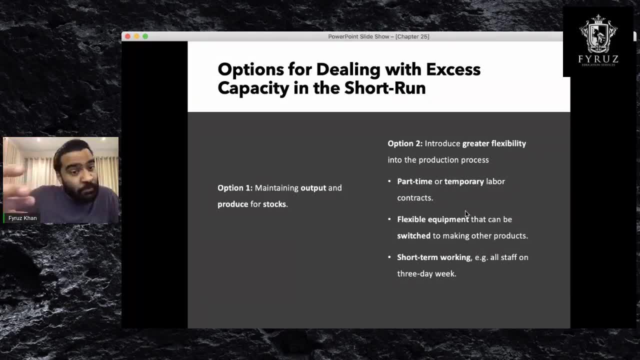 You can hire temporary staff. You can have flexible equipment. You can make other things. You can have short-term working. Instead of working for seven days, you can just work for three days Or four, Four days. Okay, That's what you can do. 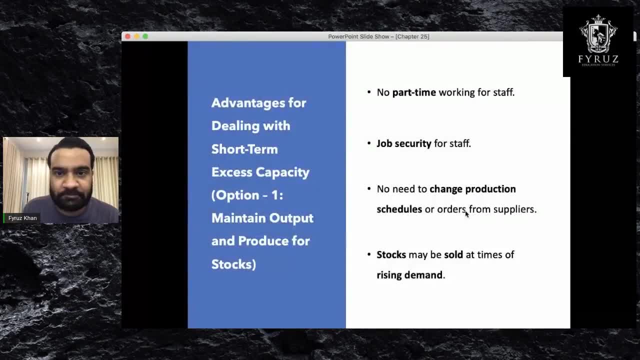 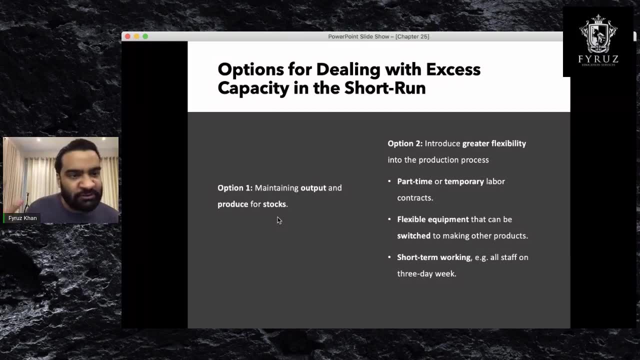 So, yeah, there we go. So we will have a look at. you know advantages of this. If you just don't think about anything, if you just don't care about anything, and if you just produce, let's say, clothes or food for 150 people, what happens? 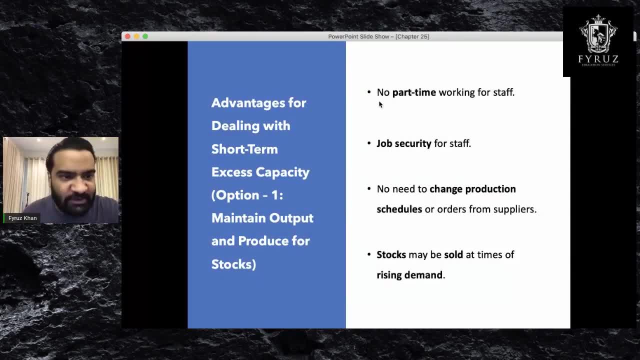 You don't need part-time staff. Everybody will be motivated, Everybody will have job security. You don't need to change production schedules And you know you make stocks and stocks can be sold later. So let's say I don't have demand for these kind of diaries now. 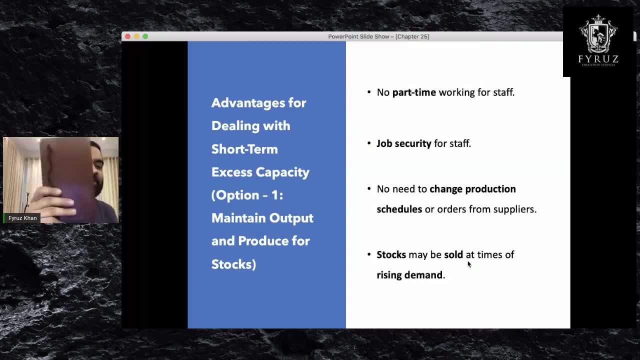 but there will be demand after three months. So I will just keep on producing And I will store it in a warehouse and I can sell it later. So there is no point of changing my production line, There's no point of, you know, changing 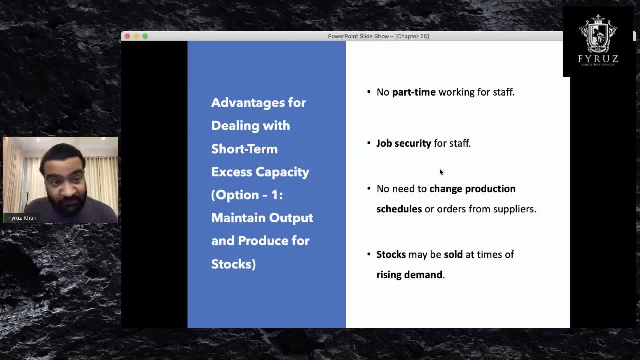 There's no point of changing my- you know- workers or getting rid of them. No, I don't need to do that. Okay, I can just produce. This is a diary. I can store it. If it was food or drink, I would think about it, because those are perishable goods. 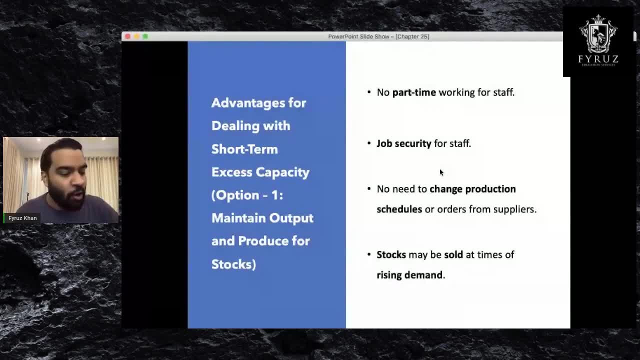 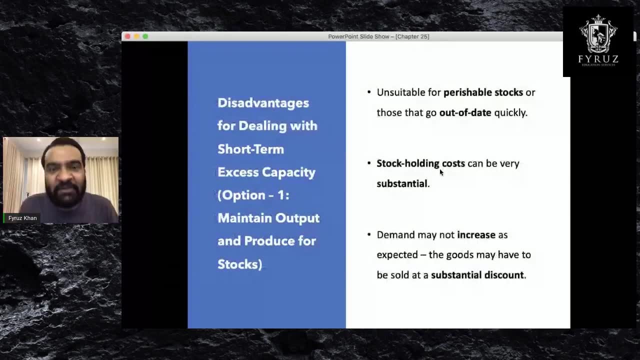 Since it's a diary or since, let's say, it's a phone or a pen, I can store them. So I will store it. I will make it and store it. Okay, But the disadvantage to that is it cannot be used, as I told you. 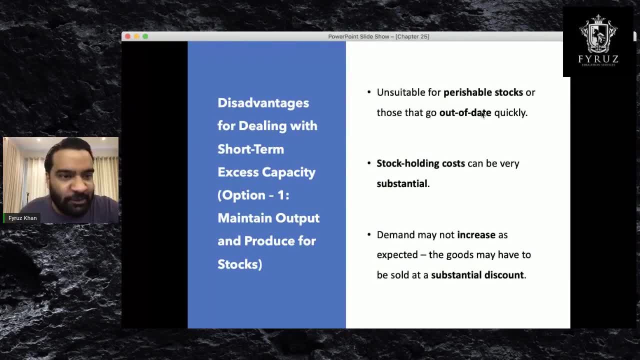 it cannot be used for For perishable stocks. it cannot be used for I'm having a grape juice. It cannot be used for a grape juice. It cannot be used for fruits. It can be used for frozen food. And then also, you have to keep in mind about your stock holding cost. 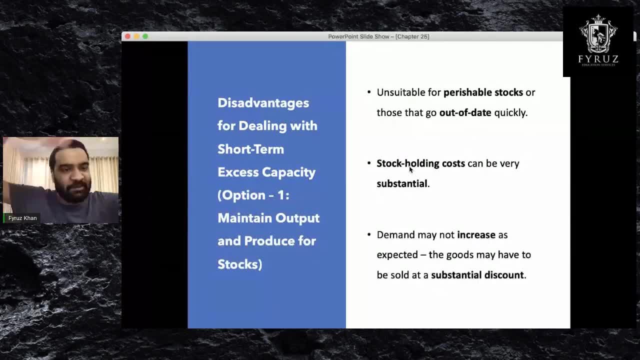 When you hold stocks, it increases your cost because you need a warehouse to store them, And that may increase your cost substantially. Okay, And let's say I'm storing this item, but demand may not increase. There's no guarantee that demand will increase for this. 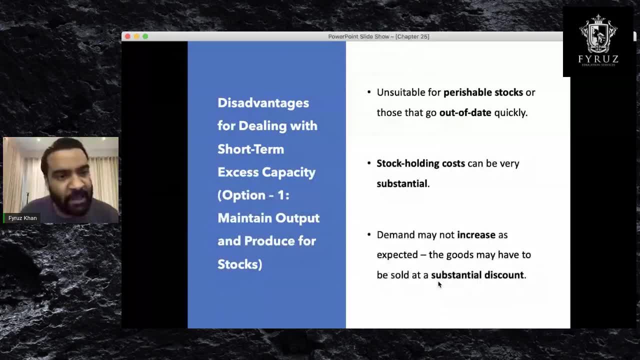 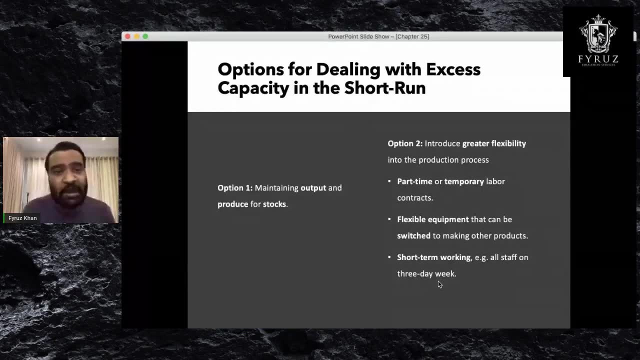 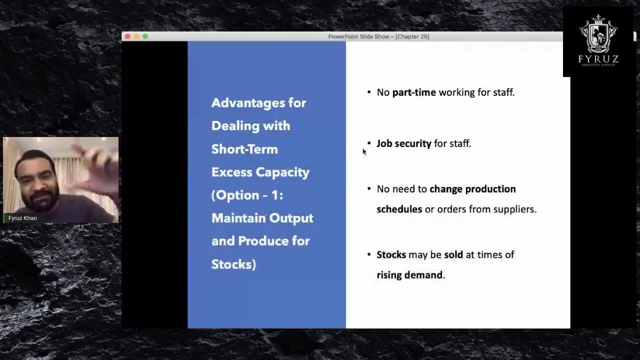 There is no guarantee And the goods may also get damaged. So these are the advantages and disadvantages for option one. When you have excess stock, what you can do is you don't care about anything, Just maintain output and produce for stocks. These are the advantages. 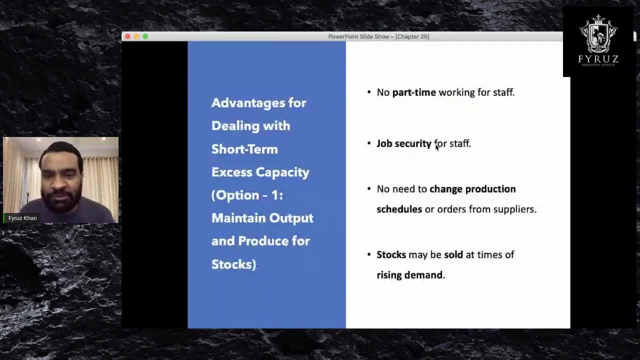 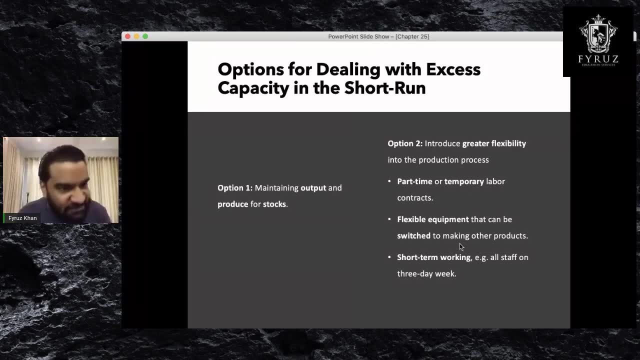 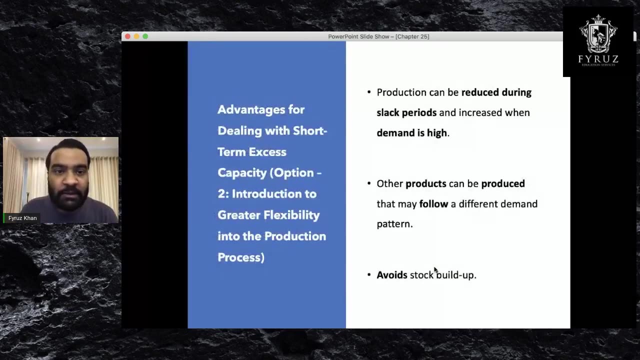 Okay, And these are the disadvantages. But if you go for option two, if you have excess capacity, option two is hiring part-time or temporary labor, having flexible equipment and producing something else rather than your main product, short-term working conditions. So the advantages is that you know production can be reduced. 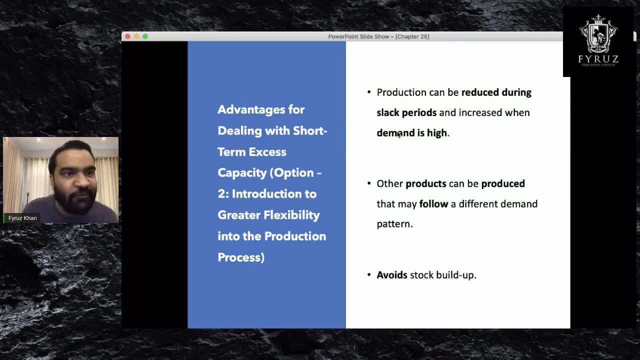 You can reduce your production, So you're not going for waste. You're reducing waste, Okay, And other products can be made. So now let's say nobody is having, let's say nobody is using, let's say, headache medicine. 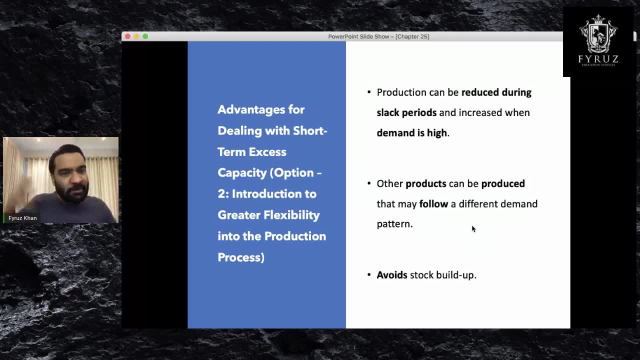 But now everybody is using sanitizers. So let's say we're a pharmaceutical company To make sanitizers- it's so easy. So instead of making other medicines, we will focus on sanitizers. We'll focus on making medical gloves and masks, because they are being sold. 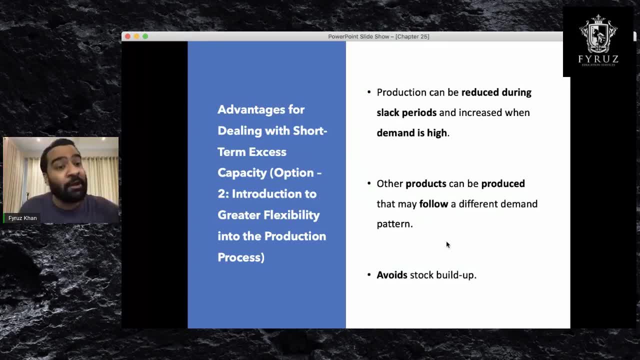 Right. They are in huge demand, So we can make other products if we have flexible machines And it avoids stock building up, because when you build up stocks, there is no guarantee whether you can sell them in the future or not. There is no guarantee as such. 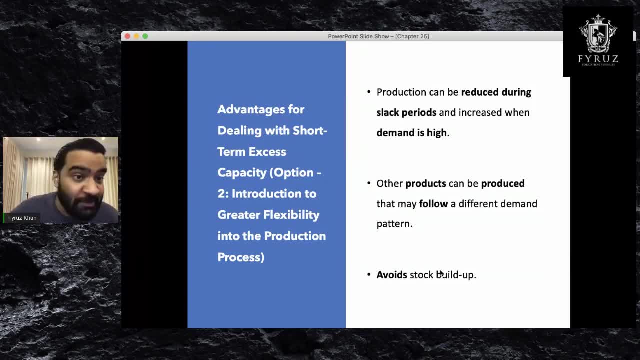 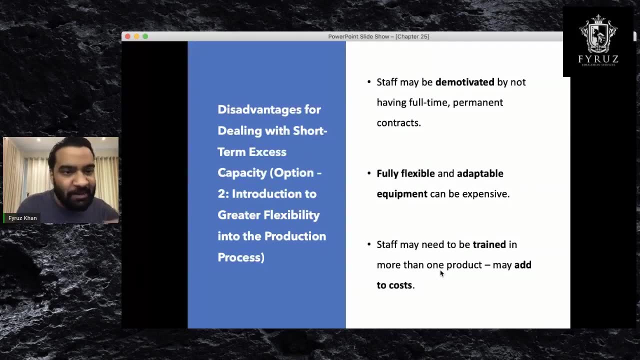 Okay, Costs will rise. Goods may get damaged. What do you do then? But, however, the disadvantage is that staff may be demotivated because you will make them temporary workers. You will call them whenever you need. You will probably get rid of them, make them redundant because you don't have orders. 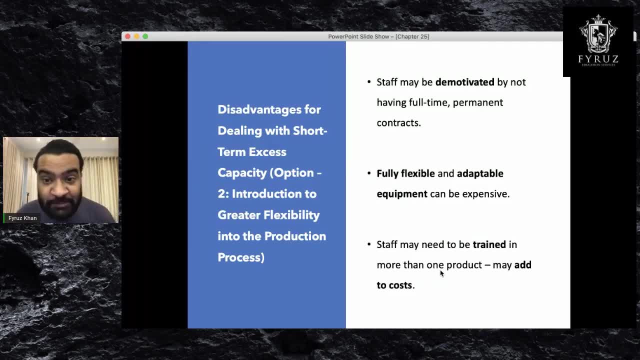 Then having fully flexible machine can be very, very expensive. So what do you do then? If you fully flexible machine means active machine, do it in the product. So those kind of machines are quite expensive, Right, The third: staff need to be trained to use. 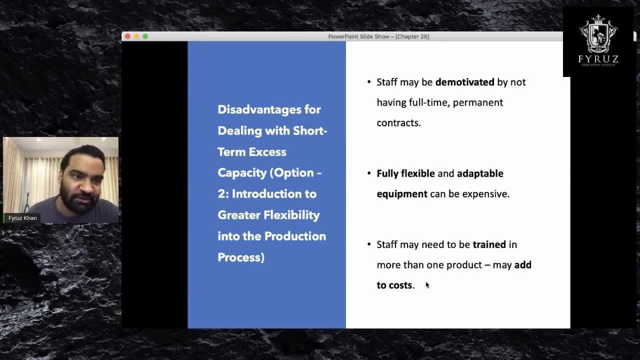 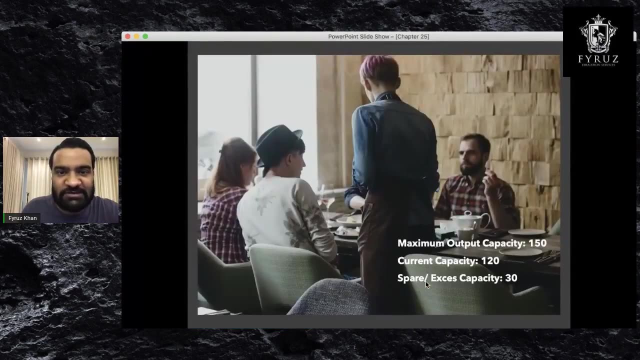 Those kind of machines And it may add to the cost. Okay, So there you go, We'll stop here And we finished quite quickly. We finished smoothly, 25 minutes in. So today's chapter was about this: capacity utilization, Okay. 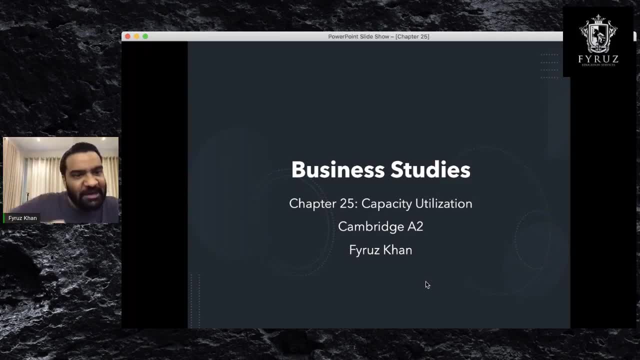 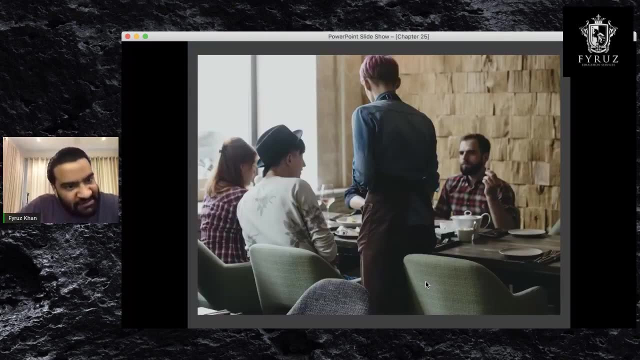 Capacity. utilization means how much capacity are you using compared to your full capacity? Okay, Okay, Compared to your maximum capacity. I've given you an example of a restaurant. Okay, Let's say a restaurant can have 150 customers now, but every day you feed 120 customers. 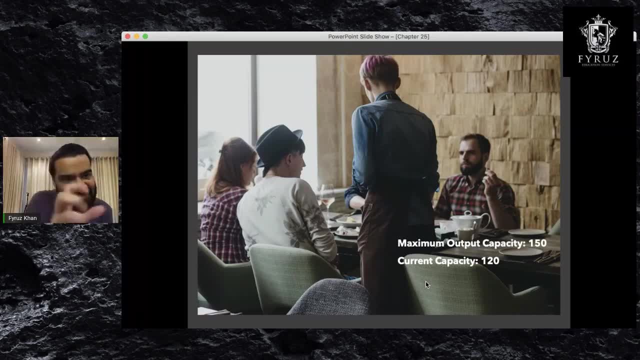 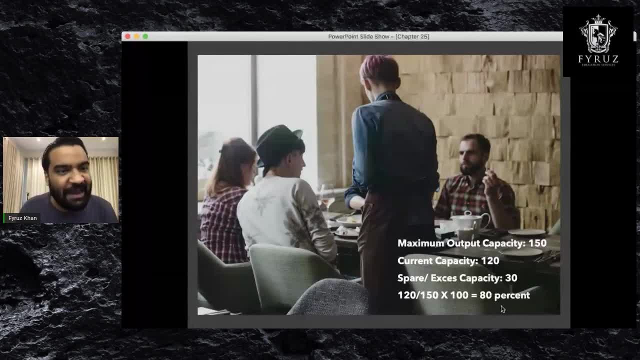 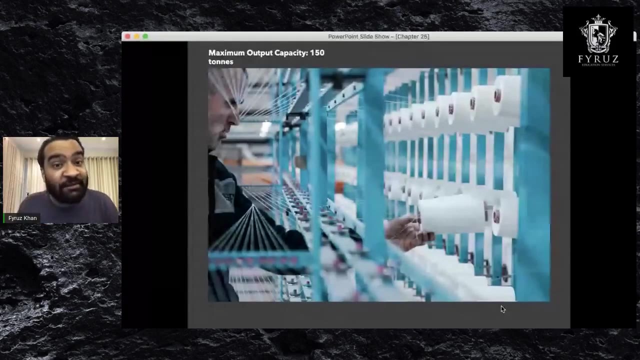 Okay, Okay, Okay, Okay Okay, Let's have a look at a factor. Let's have a look at a factor. So if we have a maximum output capacity, it's 80%, But they're not producing at full capacity. 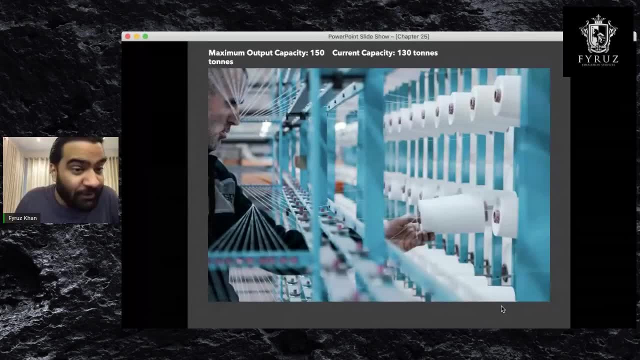 Okay, They're producing at 130 tons, which is very, very good. Spare capacity is very less: 20.. Just 20. Okay, And if you want to find the rate of capacity utilization, 130 divided by 150, into 187 percent, this is a good amount. but running at full capacity is good. 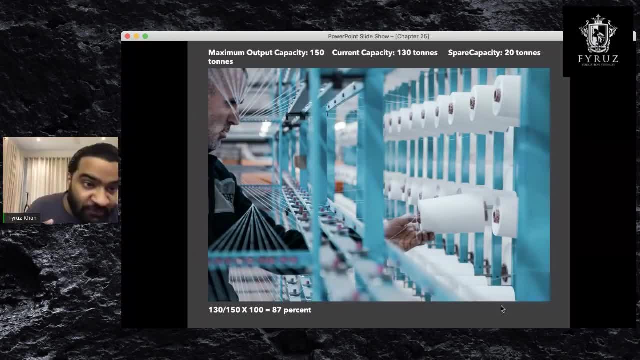 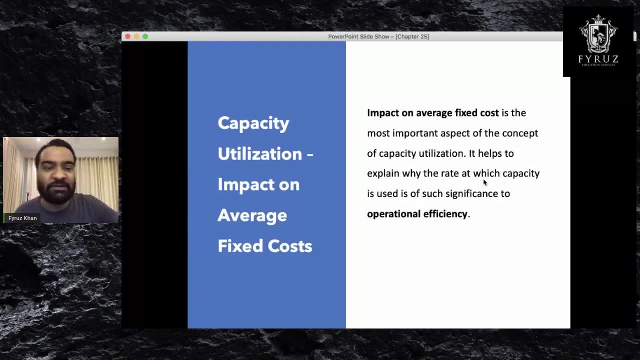 if you have 150 metric tons, if you can produce 150 metric tons, that's an advantage. okay, yeah, the formula is here. there you go. so that's an advantage because your average cost will fall. it'll have an impact on your average cost. the more you produce, the better it is for you, okay. 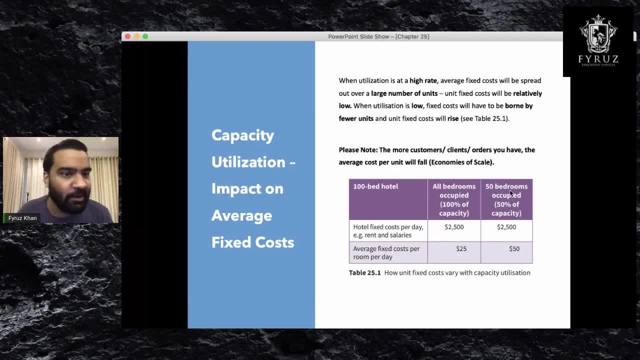 we've also seen an example of a of a hotel. let's say a hotel has a hundred room. now the fixed cost of the hotel is two thousand five hundred dollars. when you have all hundred rooms booked, your average cost is just twenty five dollars. but then when only 50 percent of it's booked, then your 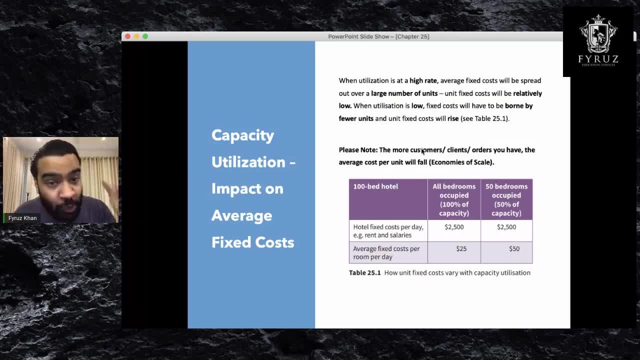 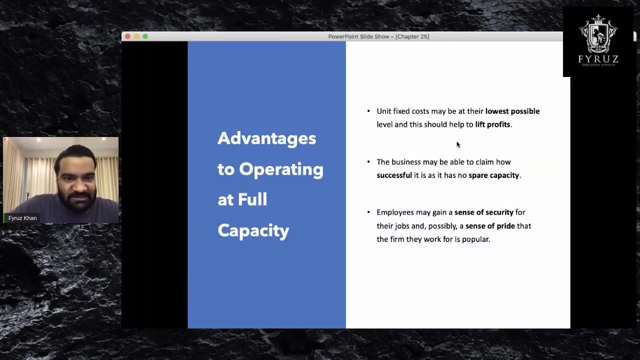 average cost rises to fifty dollars. so note that the more customers, the more clients, the more orders you have, your average cost per unit will fall and that that is economic scale. okay. what are the advantages of running at full capacity? there we go low cost. you'll feel successful, you'll have sense of security, sense of pride, drawback staff. 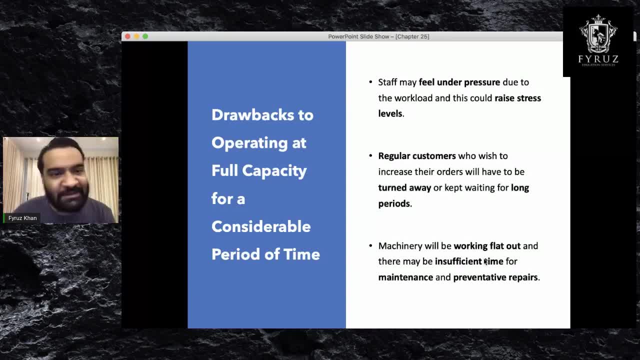 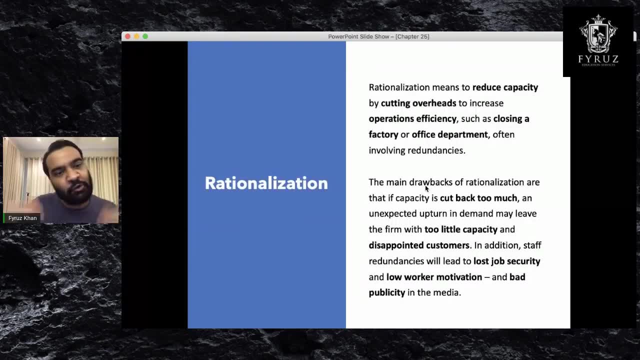 may be under pressure. machineries will be working 24: 7 and that's not good. and regular customers may be turned away- okay. and we've talked about excess capacity. we've talked about rationalization, cutting down off extra cost or overhead cost, shutting down factories- uh, making workers redundant? okay. and when you have excess, 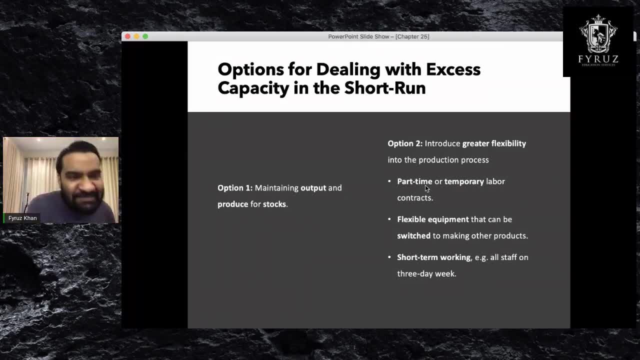 capacity. let's say you have 150 tons, but you're producing at 80- 90 tons, so that's not a good average. so what should you do? so you have two options: you can maintain your uh, your current uh stock level, which is your 150, and you can stock the items and sell it later, or you can take option. 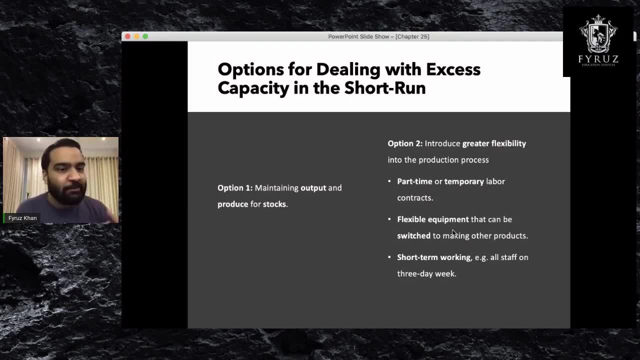 two. uh, you know, get rid of everything. you can get rid of everything. you can get rid of everything. employees, or make them part-time or temporary. for a full time, uh have flexible equipment and produce something else. and we've talked about the advantages and disadvantages for both the options. 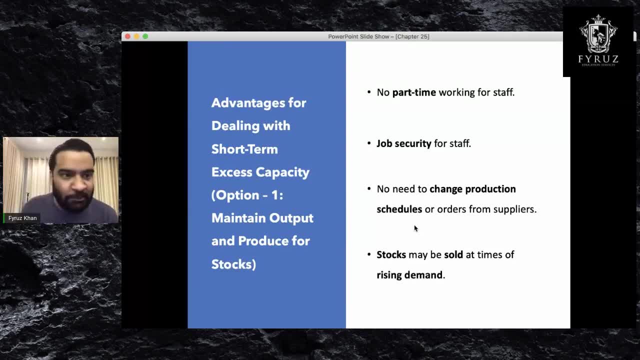 right, so we will stop here. it was a great class. we finished half of this chapter. tomorrow we'll finish the whole chapter and and yeah, we'll be done with this chapter. so great. thank you very much. i will see you again. if you have any comments, do not forget in the comment section.